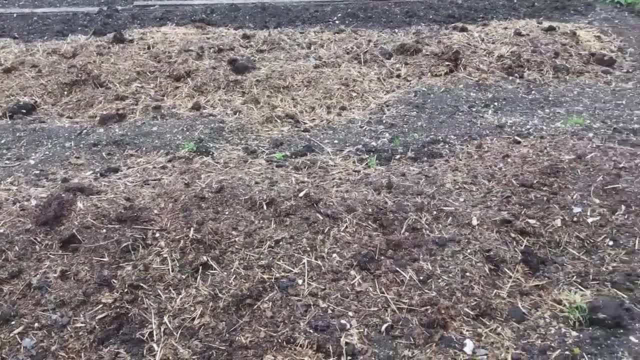 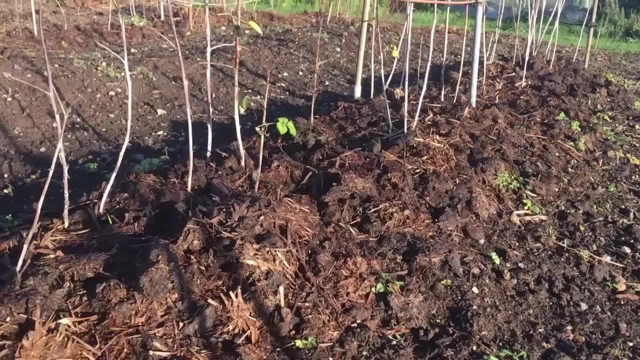 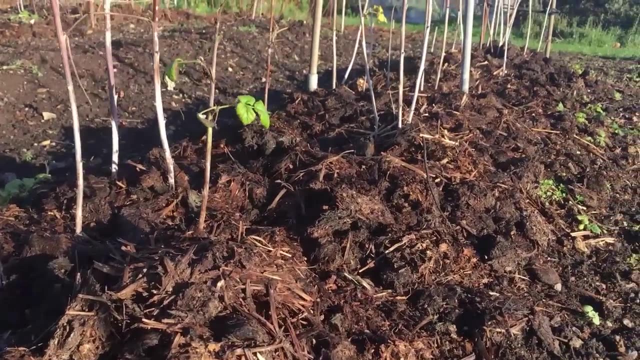 and may burn plants due to its very high nitrogen content. Add organic matter whenever you can and at least once a year. This can be simply laid on the soil surface as what's known as a mulch. Over time, your soil structure will improve, becoming better draining and a healthier environment for roots. 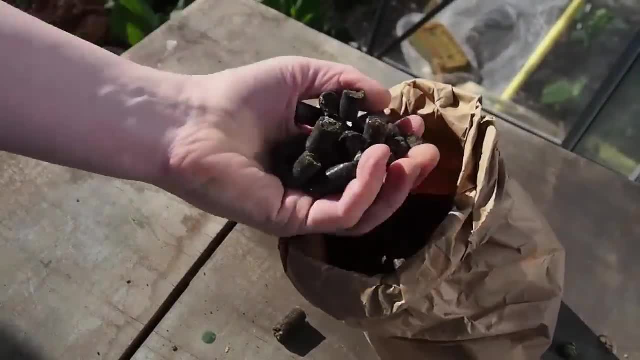 You can add organic fertilizers too, of course, but think of these as a short-term boost rather than adding organic fertilizers. You can add organic fertilizers too, of course, but think of these as a short-term boost rather than adding organic fertilizers. 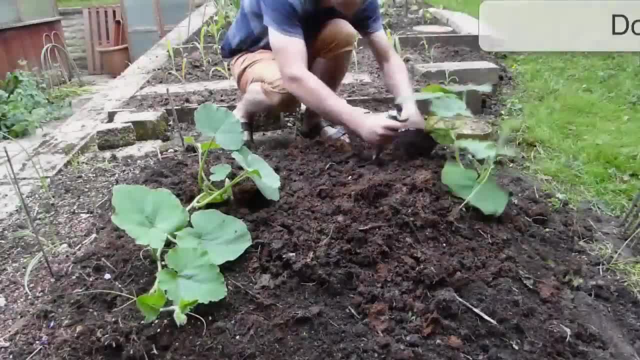 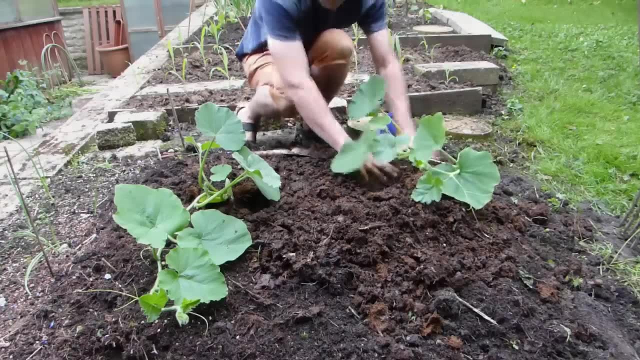 You can add organic fertilizers too, of course, but think of these as a short-term boost rather than adding organic fertilizers. As a new gardener, it's easy to get carried away, but a little restraint is essential. Plant too soon and tender plants are likely to be caught out by a sudden frost or will fail to thrive as they grow on. 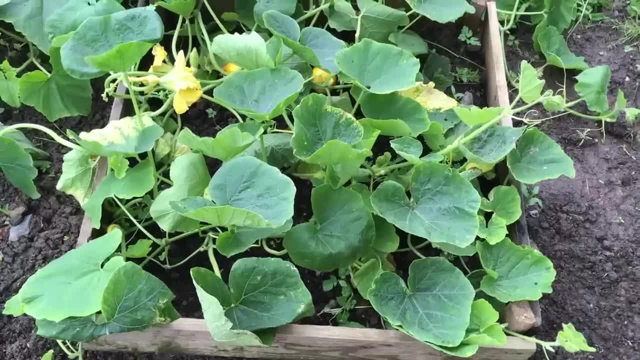 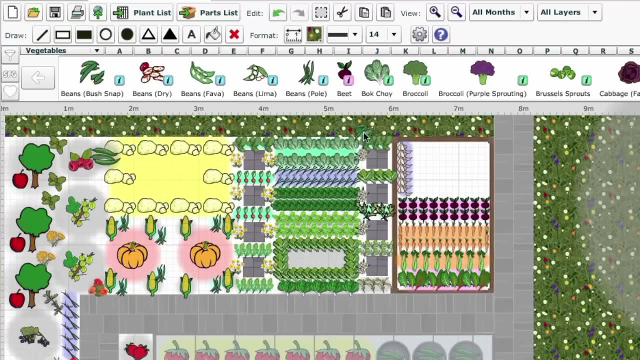 In most areas. your last and first frost dates define your growing season. Our Garden Planner can help. It automatically calculates your frost dates based on your location. As you add to your plan, the accompanying frost dates will be calculated based on your location. 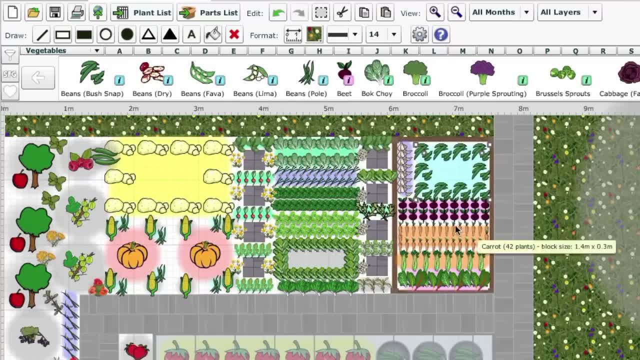 As you add to your plan, the accompanying frost dates will be calculated based on your location. As you add to your plan, the accompanying frost dates will be calculated based on your location. Open it up and you'll be able to see exactly when you should be sowing, planting and harvesting your chosen crops. 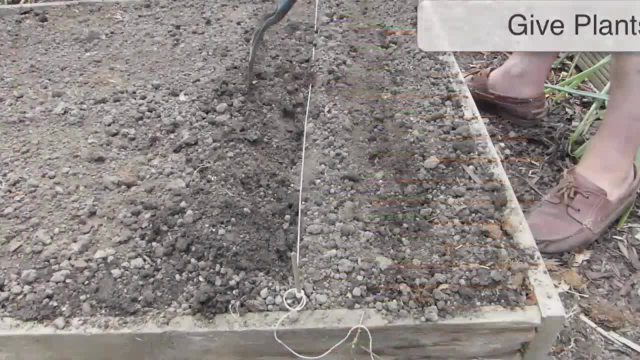 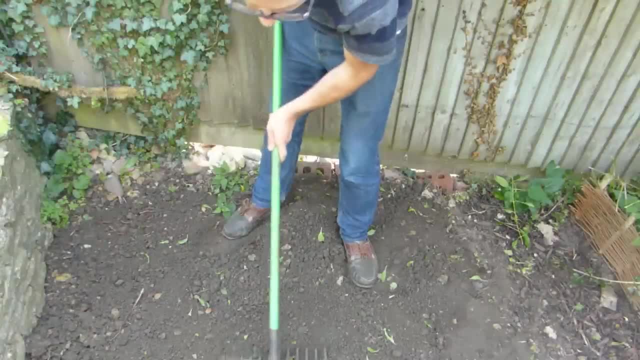 Open it up and you'll be able to see exactly when you should be sowing, planting and harvesting your chosen crops. Begin sowing outside only once your soil has warmed up and dried out enough to become workable. Seed beds should have a fine, crumbly texture. 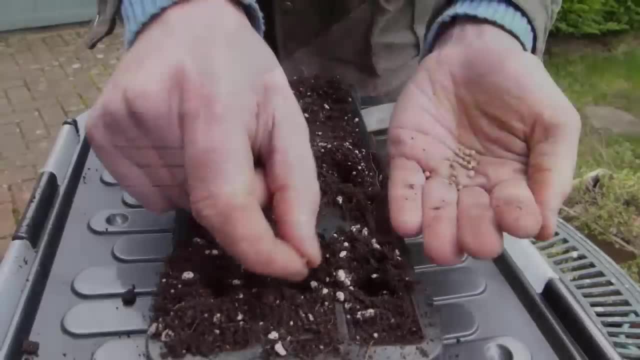 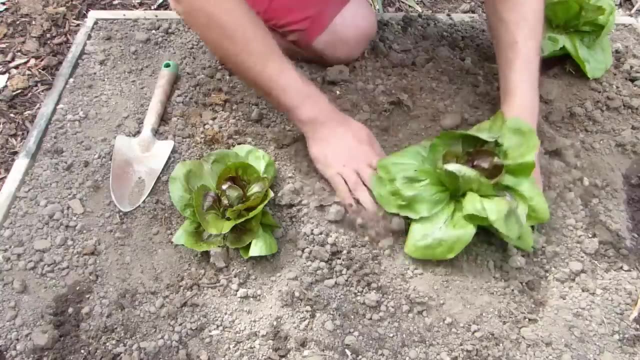 Sowing undercover into plug trays and pots is a great way to get a head start while temperatures outside are still too low. Transplants need planting holes that are bigger than the existing root ball. The soil then used to fill in the hole will be looser. 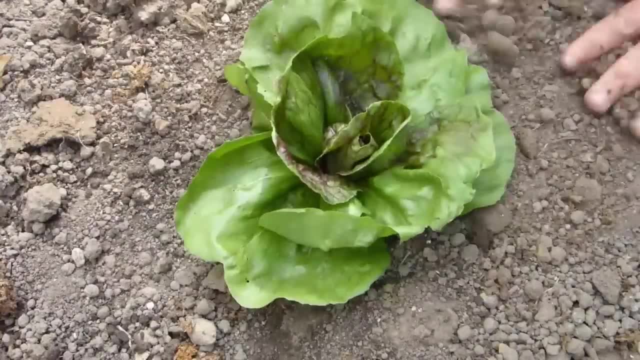 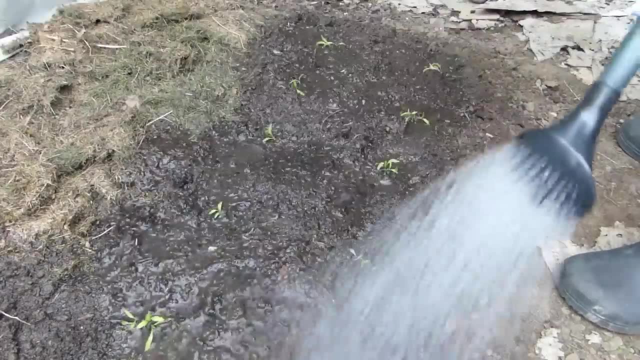 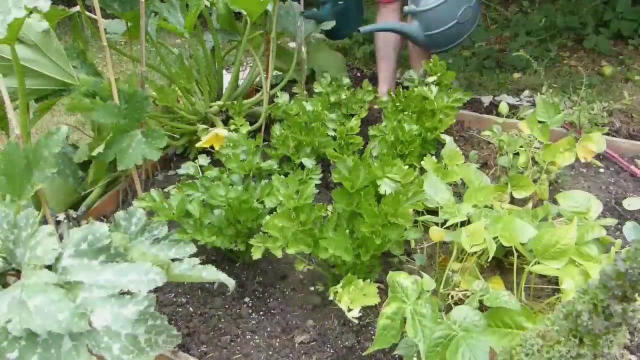 which will make it easier for new roots to grow out into the surrounding soil and help plants to establish quicker in their new home. Most plants need an average of 1-2 inches or 2-5 cm of water a week. You'll probably need to water more as it gets warmer, but this does depend on rainfall. 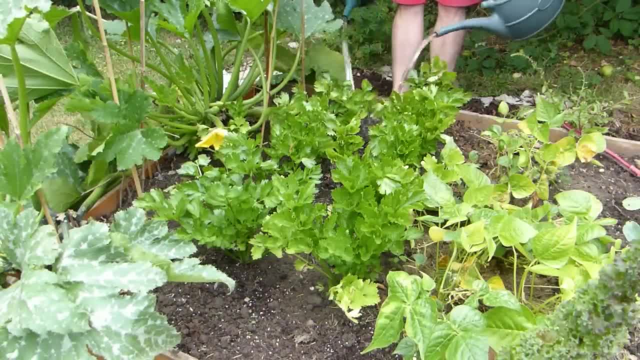 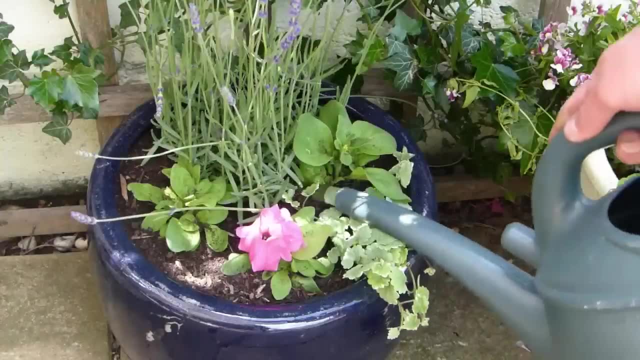 It's best to water heavily once a week than a little every day. It's best to water heavily once a week than a little every day. This forces the soil to absorb more water. This forces roots to reach further down into the soil to seek moisture, improving self-reliance. 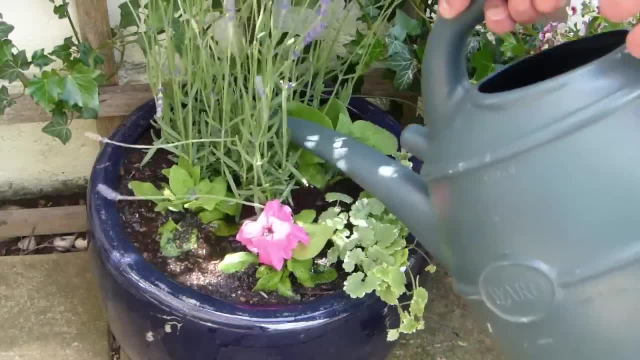 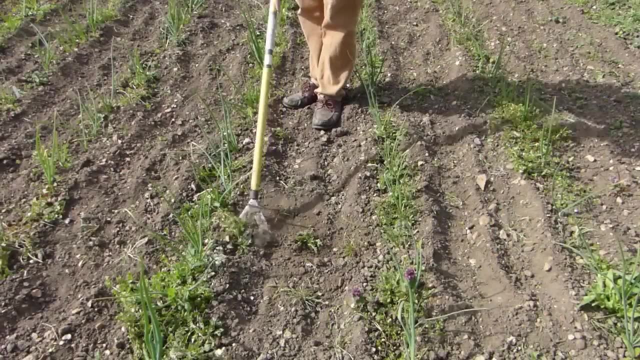 Planting containers can't do this, of course, so water them more often. Remove weeds as soon as you see them, so they don't have a chance to produce seeds and spread. Hoeing is quick and easy, and severed weeds may be left where they fall to wither in the sun. 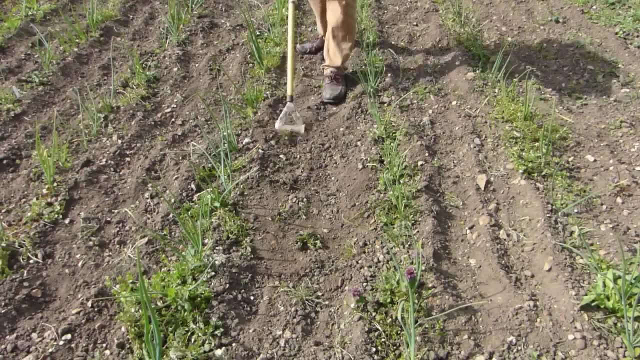 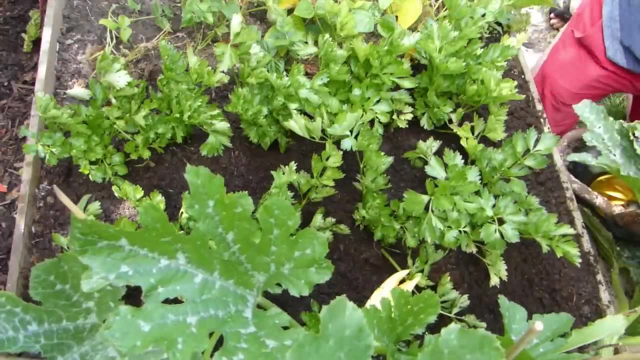 Keep the blade edge sharp and close to the surface to prevent damaging crop roots. Handweed where the hoe can't reach. Mulching with organic matter is a great way to stop new weeds popping up, as well as improving your soil as it gradually rots down. 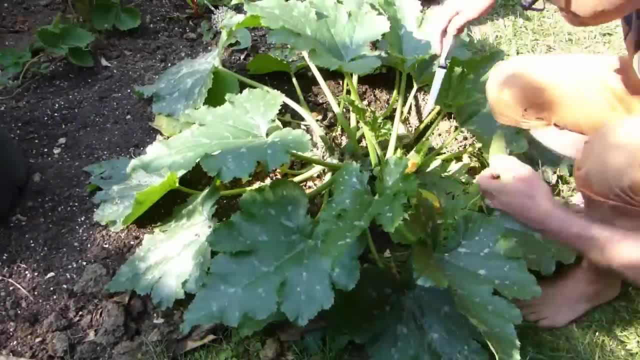 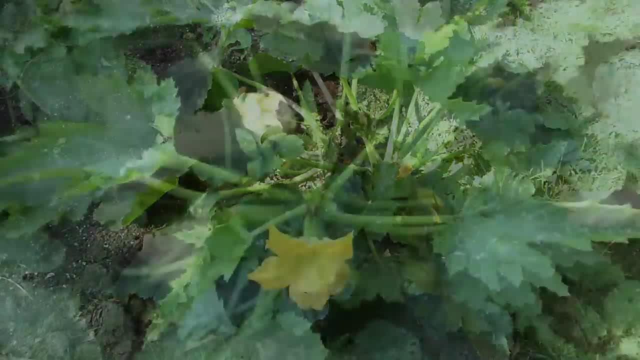 Some vegetables must be picked regularly to keep the harvests coming. Beans, zucchini or courgette and tomatoes are just a few examples where picking will encourage even more pods and fruits to follow. Similarly, removing old blooms from flowers called deadheading. 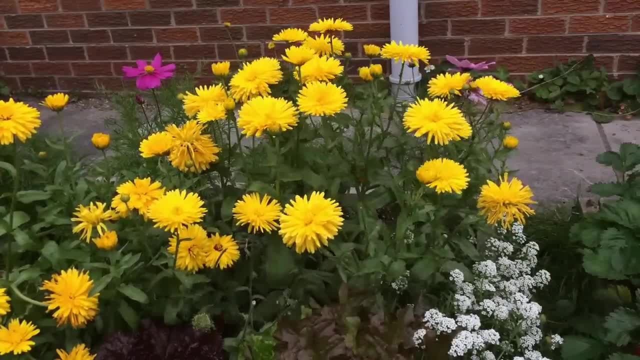 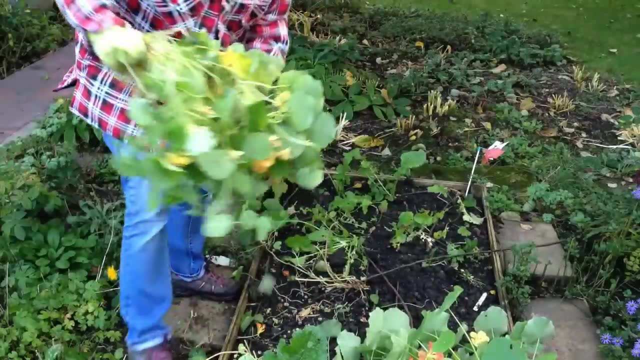 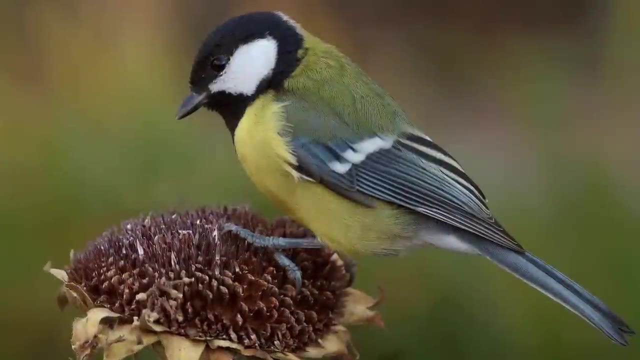 encourages more to follow extending the display a little longer. An end of season tidy-up is a great way to ensure a clean start the following year, but don't get too carried away. Old seed heads of, for example, coneflowers and thistles will help feed birds over winter. 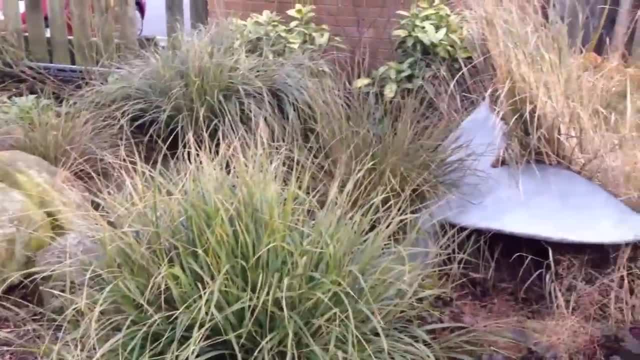 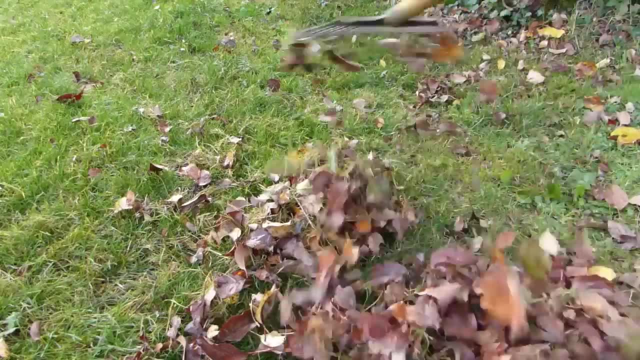 while ornamental grasses can be left to add movement and structure to the garden and overwintering sites for beneficial bugs such as butterflies. Fallen leaves are a welcome resource. Add them to compost heaps. compost them alone to turn them into leaf mould. 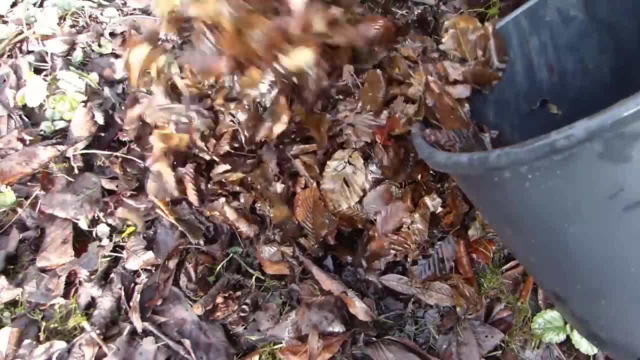 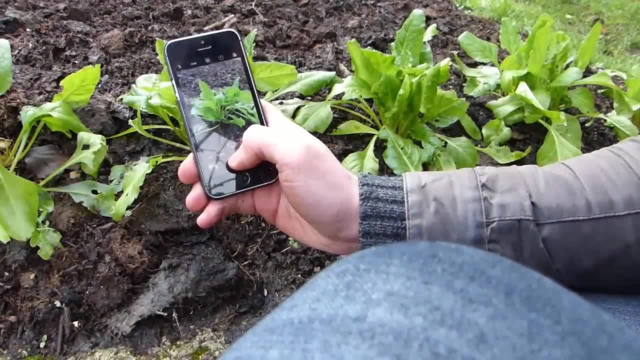 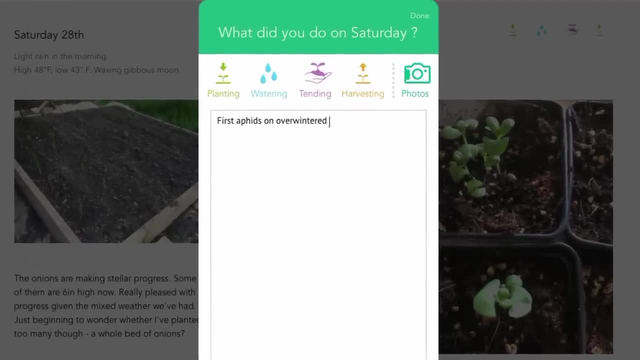 or pile them thick over tender perennials to protect them over winter. Good gardeners make lots of mistakes, but they learn from them. By keeping track of when, where and what you grew, and noting any pests, diseases or failures, you can build up a personal record of what works best for you and your garden. 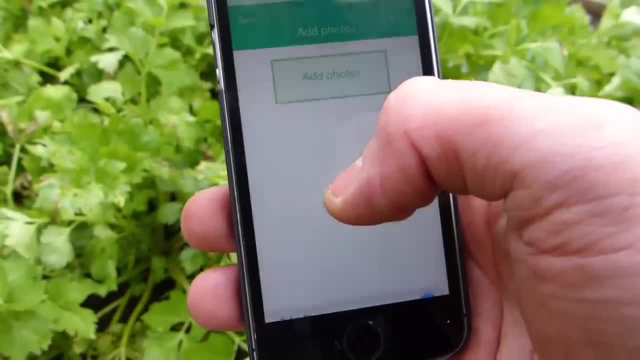 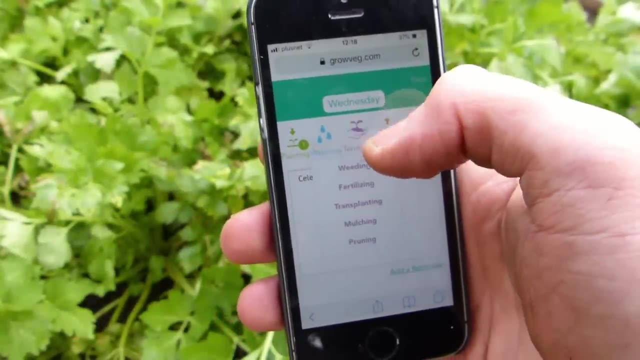 Take advantage of our free online Garden Journal, which makes record-keeping easy. Take photos outside on the go, then upload them with your written notes. notes Record when you planted, watered and tended your crops. get to the bottom of problems. 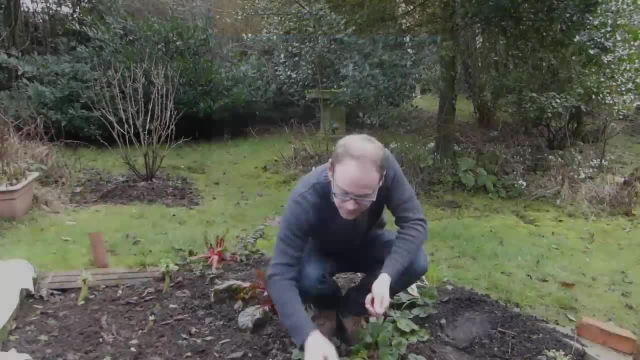 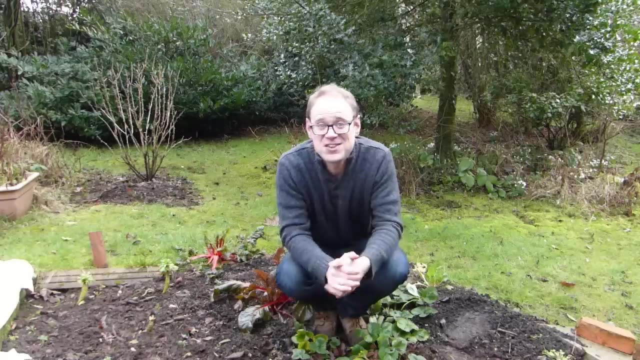 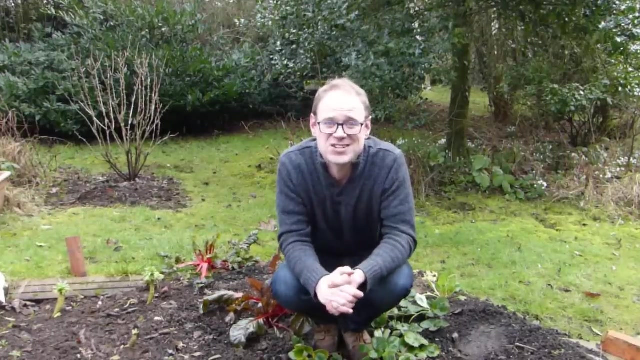 and see how much you've harvested. These tips are our recommendations, but of course, everyone has a different opinion based on their own experiences. So if you're not so new to gardening, I invite you to share your advice for beginners in the comments section below. And if you're a gardening newbie,